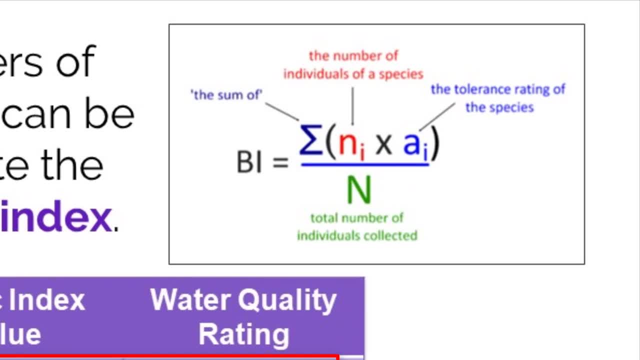 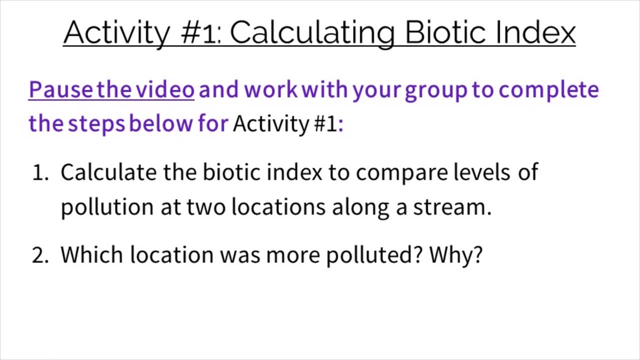 Biotic index can be calculated by using this equation. Simply put: you take the total sum of the number of individuals of a species, multiplied by their tolerance rating, and divide by the total number of organisms that were collected. This will give you a value to compare to the chart. 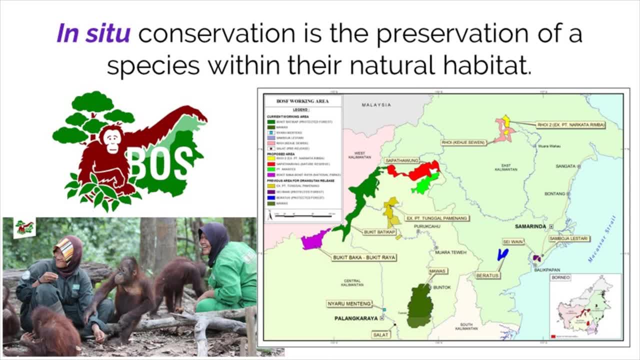 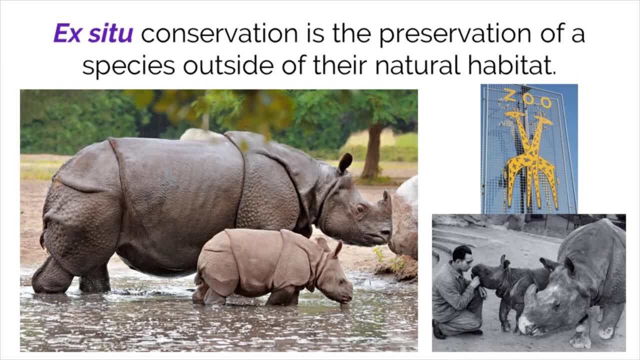 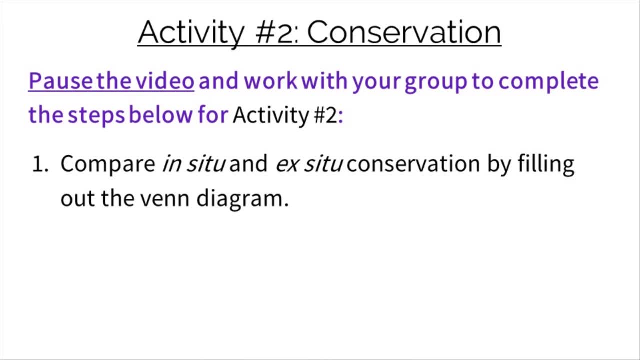 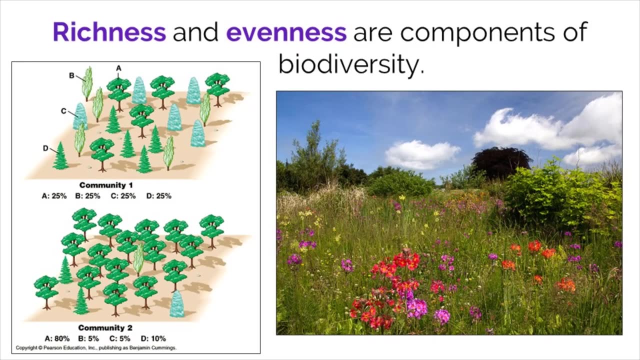 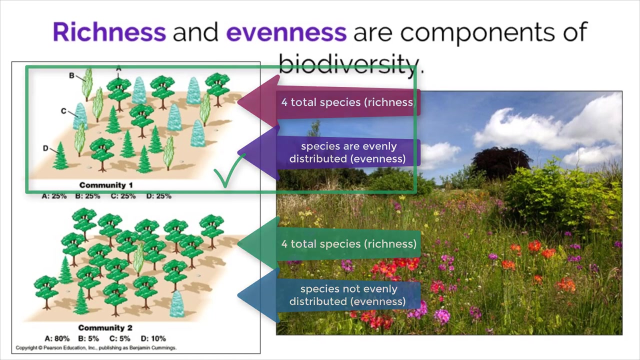 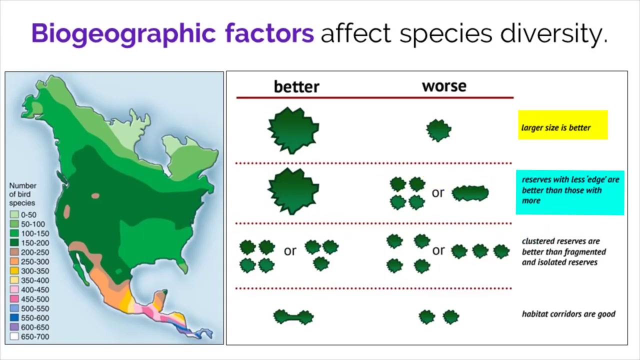 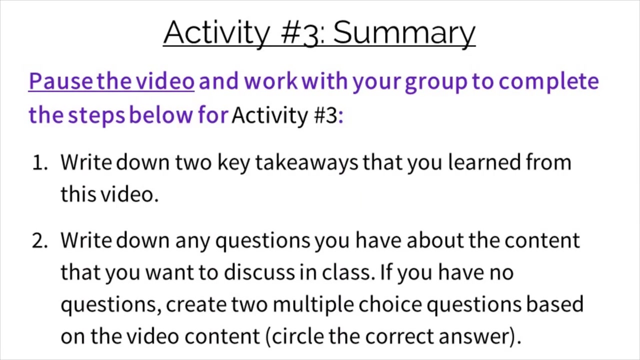 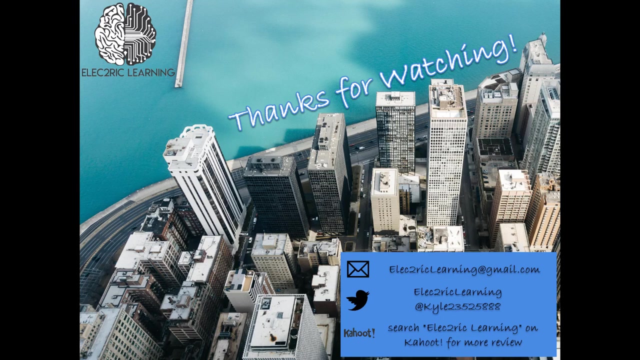